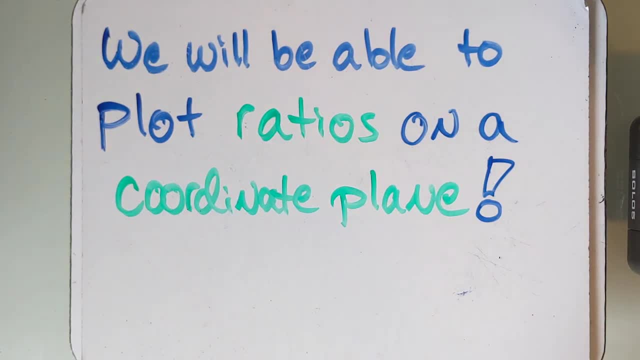 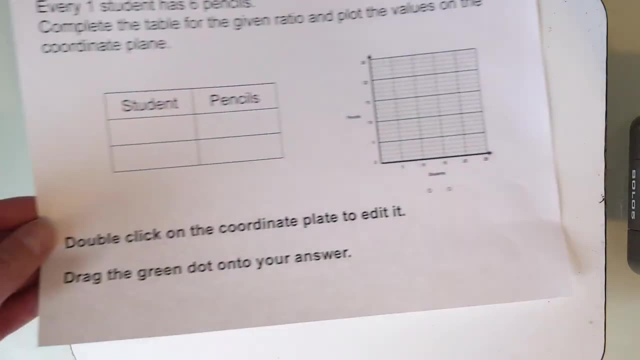 also showing our two rules of everyone tracks, so pausing and rewinding at any point, and everyone tries. Let's go ahead and take a look at our do now. Our do now today is a little bit different than it usually is. It says every one student has. 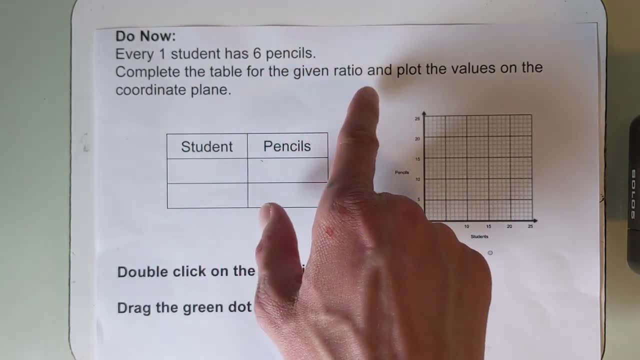 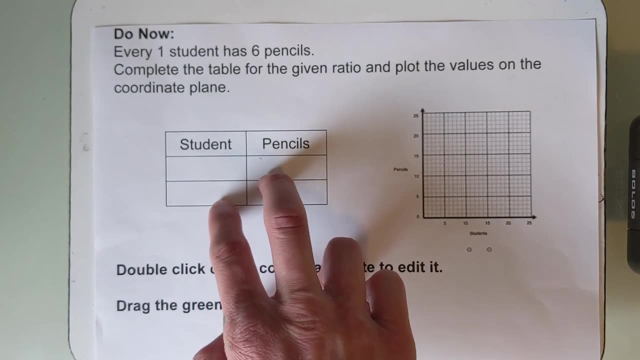 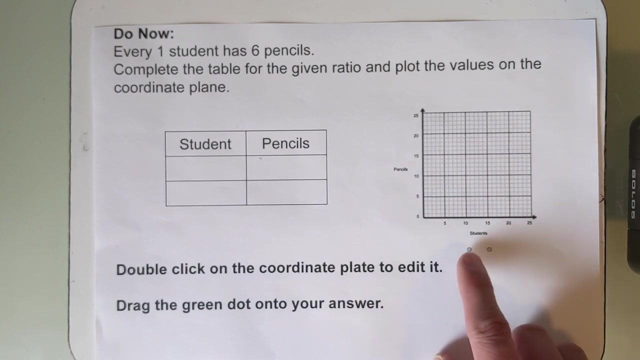 six pencils Complete the table for the given ratio and plot the values on the coordinate plane. So what that means is they want you to go ahead and fill out this table first and then double click on this in your Google Classroom and you can actually edit it. You'll have these two little. 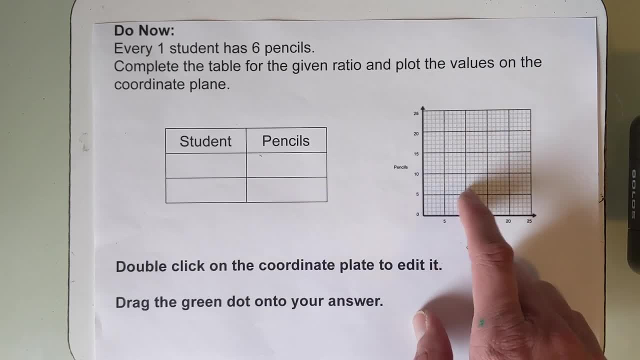 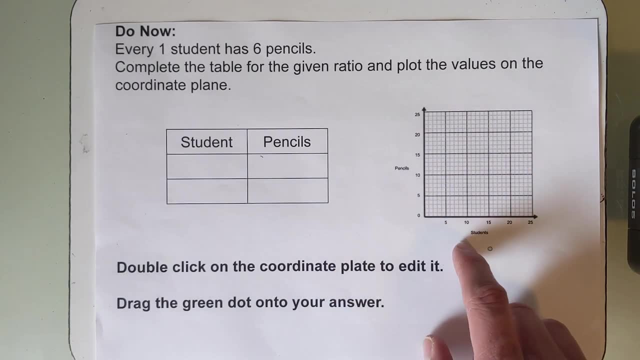 dots and I want you to go ahead and drag them to where you think they belong- on this chart or on this coordinate plane. Again, double click on this once you've filled out your table and then drag those two little green dots on to where. 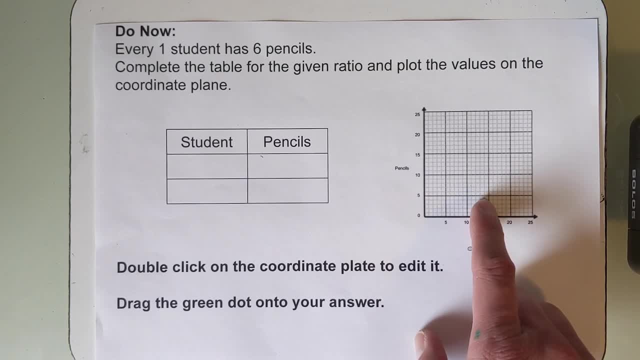 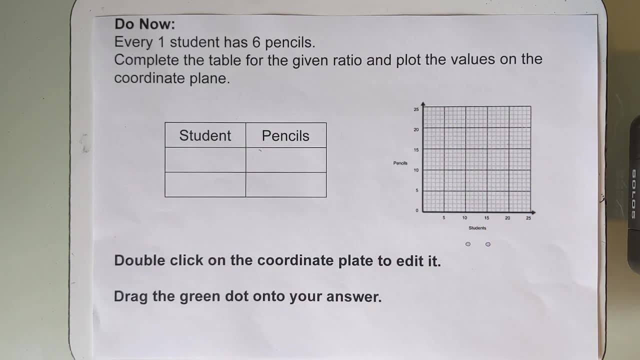 you think your answer would be: Go ahead, take as much time as you need to do this, but make sure you have this table filled out and also those two little dots moved Again. I do not expect you to have the totally correct answer, because we're 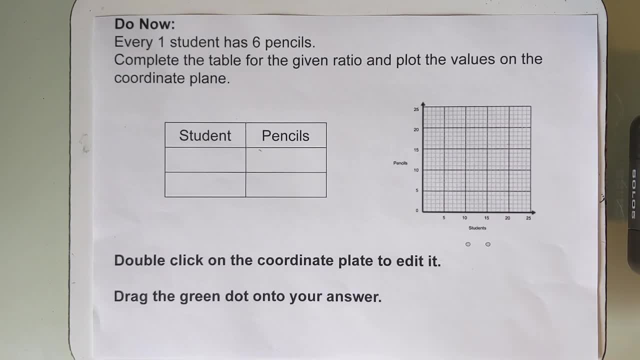 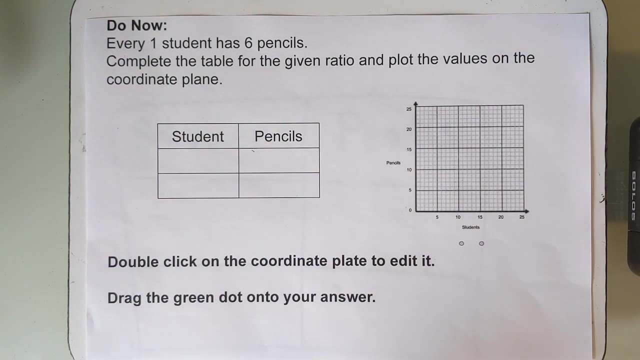 just learning this today. Go ahead and take your best. try and come back when you're ready, pausing in the next five, four, three, two and one. So at this point you've already taken the best guess on this question and you have some sort of answer written down. Let's talk. 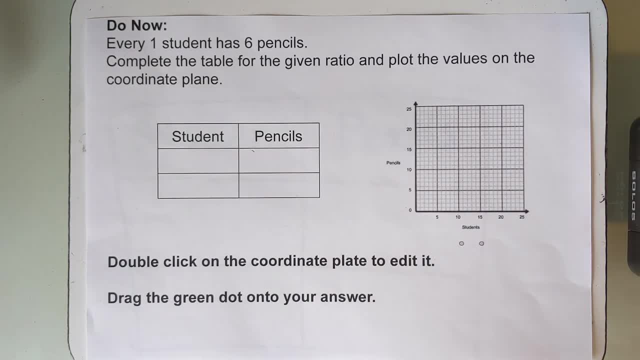 about how to actually solve it. Now, there are two parts to this question. The first part is completing this table- so with our students and pencils and our ratio here- and the second part is actually how to graph this, Or how to plot your points on the coordinate plane with your ordered pair. 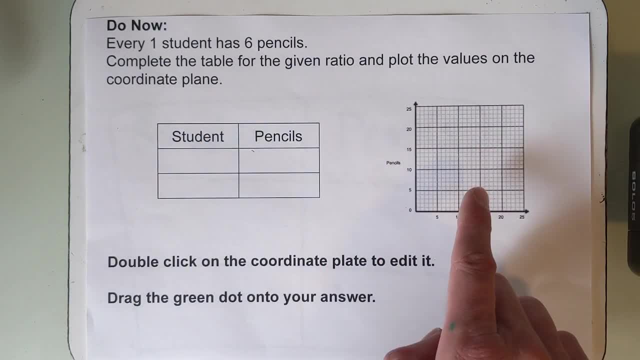 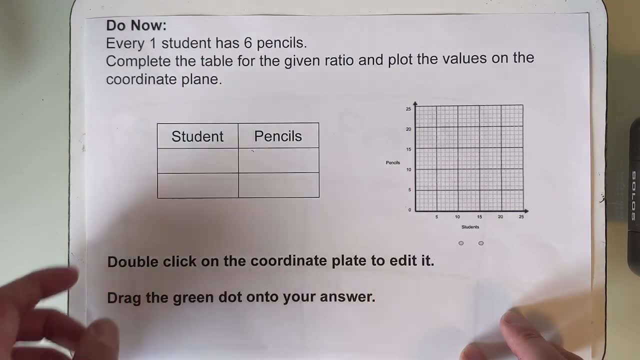 We're going to talk about the table first and then we'll go ahead and move on to this part. So again, let's talk about this table first. We know that every one student has six pencils, so our ratio here is one to six, So one student. 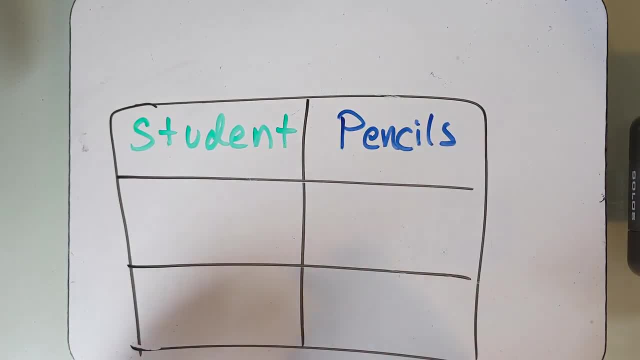 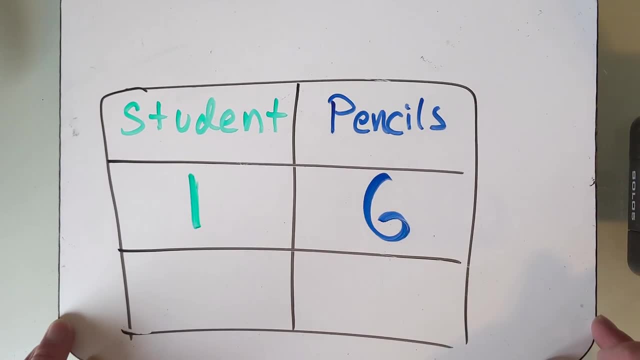 to six pencils. So in our chart I just went ahead and drew one right here we would have one student to six pencils. So it would just be one to six, Again building on what we did yesterday with our charts right. So what they're saying is: if this continues, 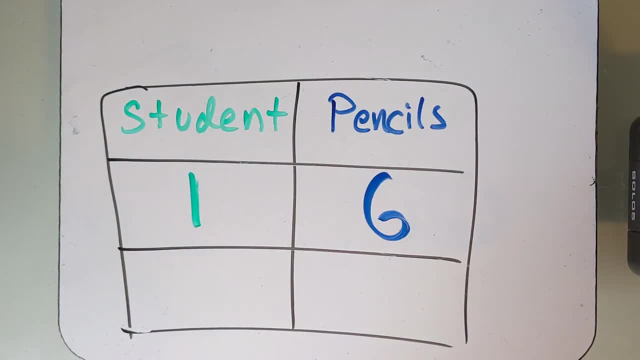 what would our chart look like? Or, sorry, what would our table look like? Now, if you notice, they don't give you anything here to write, That's okay. All I want you to do is write down what the next one would be. So for here for two students. 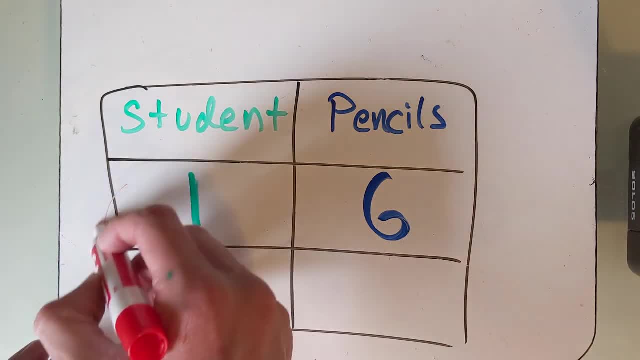 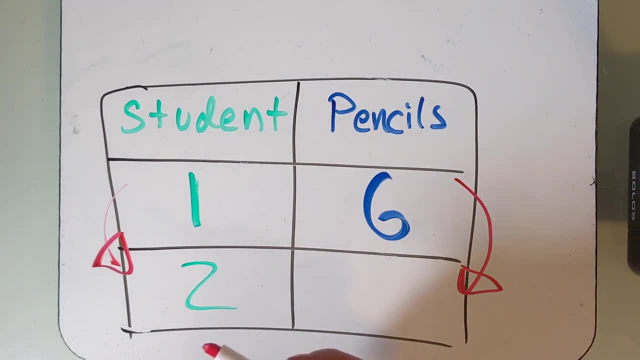 how many pencils would we have? Thinking about our rule And remembering that whatever we do to one side, we do to the other. So for here, our rule is gonna be times two. Remember we never use addition when we're finding equivalent ratios. 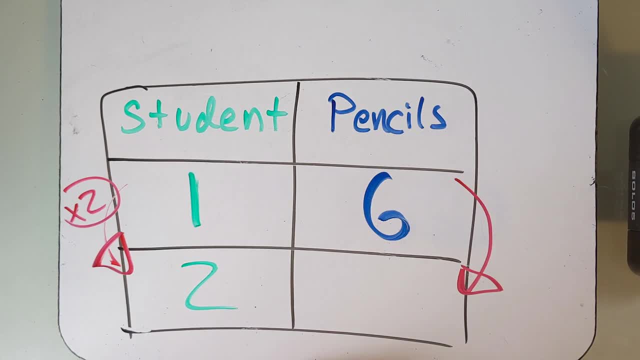 We always use multiplication, same thing with our fractions, right? So here our rule is times two. So whatever we do to one side, we do to the other. So it would be times two. So that means six times two would be twelve. So we'd have twelve pencils. So for every. 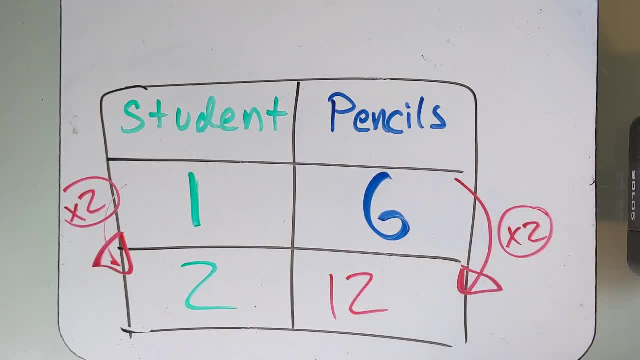 two students. there are twelve pencils, so our ratio is two to twelve. Now we're gonna go ahead and pause for a second and actually go to the computer, double click on it, the chart there, the coordinate plane- and we'll go ahead and talk about how to actually plot. 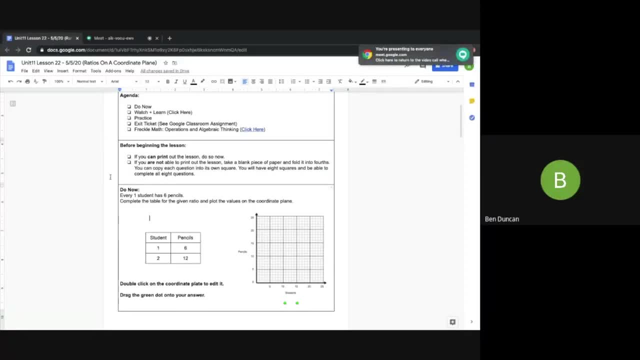 those points. So let's go ahead and take a look at how we would put our answers into this chart here. So we've already talked about how our ratio of students to pencils at first is one to six, and then the next one we would have is two to twelve. So I want to really remind 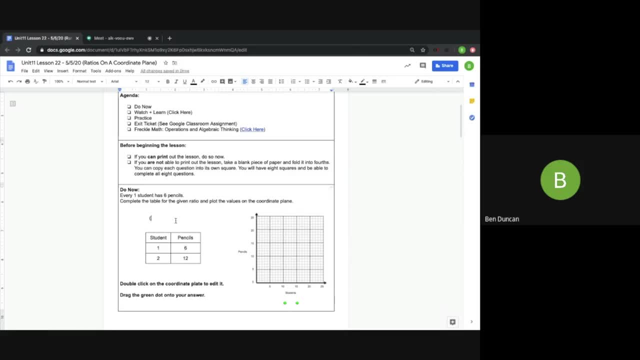 you that when we're talking about ratios like this, we can also rate ratios as an ordered pair. So it'd be one to six- it would look something like that, And then our next one would be two, And this is how we would rate it: two to twelve. So when we think about how to plug in an ordered 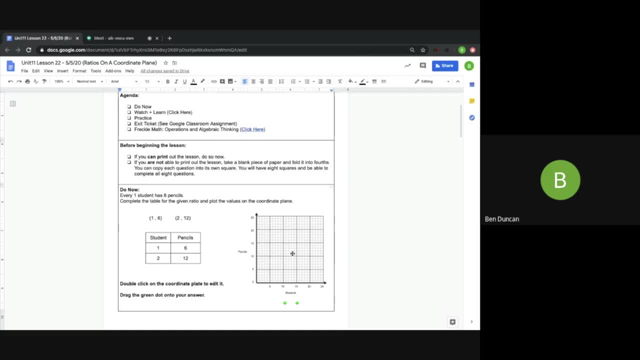 pair onto a chart or a graph. we just go ahead and plug it in the way it's written. So remember, we go over and then up. So we're gonna start with a one to six In order to do that and edit this. what we're gonna do is double click on it and it's gonna bring this up And what? 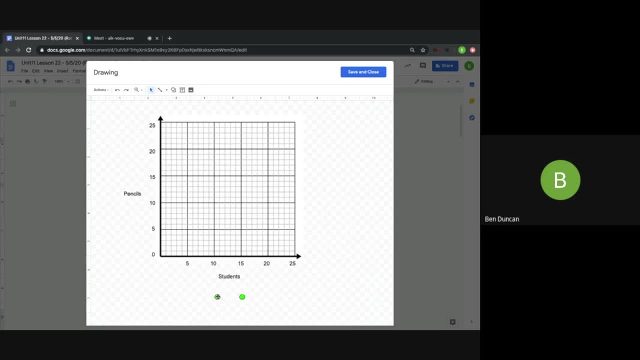 you can do is you can take these two green dots and we're gonna place the first one on one to six, So we start at zero. So again, just kind of drag it around: We start at zero, go over one and up six. We're just gonna drop it right there And then the other one. 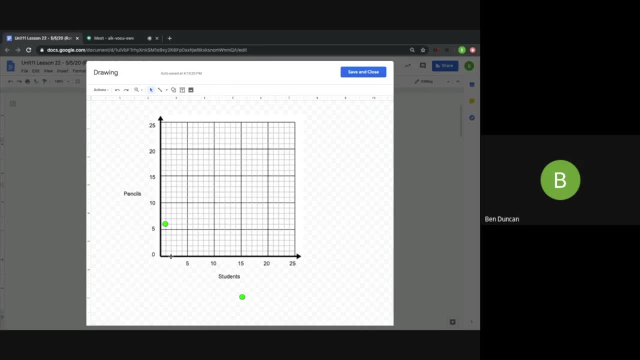 was two to twelve. So we're gonna go over two and up all the way to twelve right up here. So let's go ahead and do that. So we have our two to twelve up to twelve right here, And then we just leave it. So what we would do is we would just press save and close. 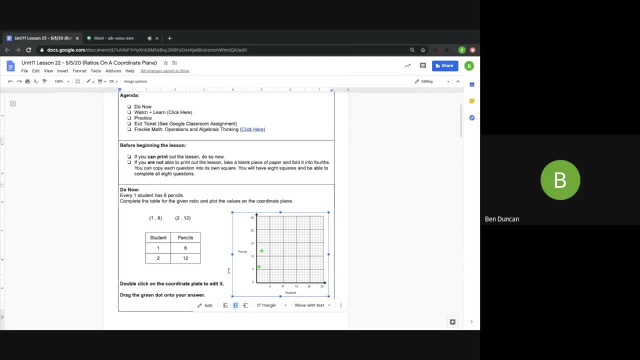 And now those are marked right there. So that's how we'd put these in. So our first ratio again is one to six. So one to six is marked right there. And then two to twelve, Again just over two and up twelve, Remembering that we already did this during the school. 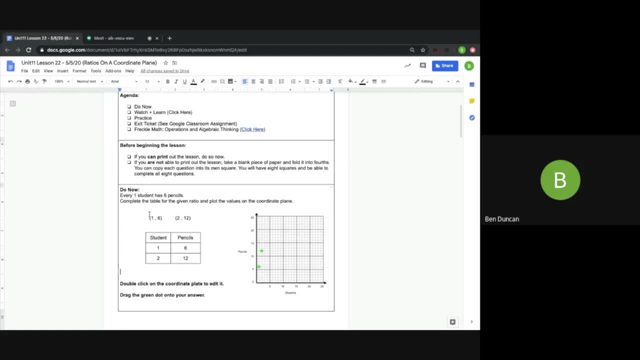 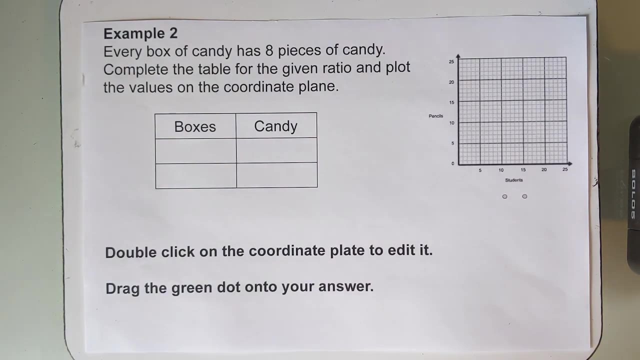 year. Remember you have to walk before you can jump right, So you have to walk over to the over and then up up to six. Let's go ahead and take a look at the next question. Nice job, guys. So we took care of our first example. Let's go ahead and do one more. just 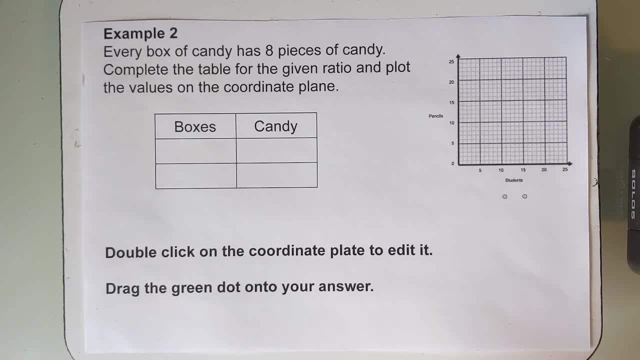 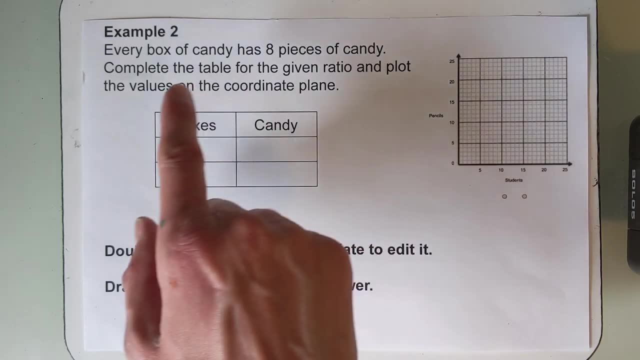 to make sure you fully and really understand what's going on. So for question number two, it says every box of candy has eight pieces of candy. Complete the table for the given ratio and plot the values on the coordinate plane. So we already have our table set up. 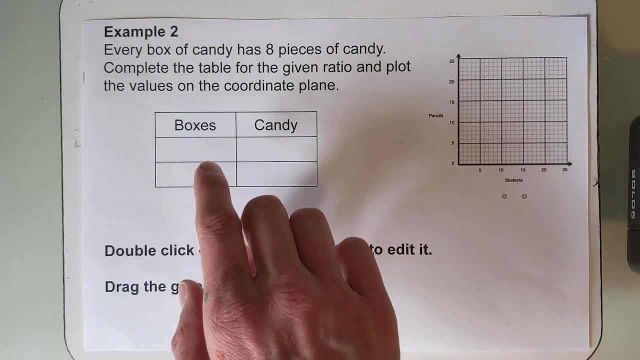 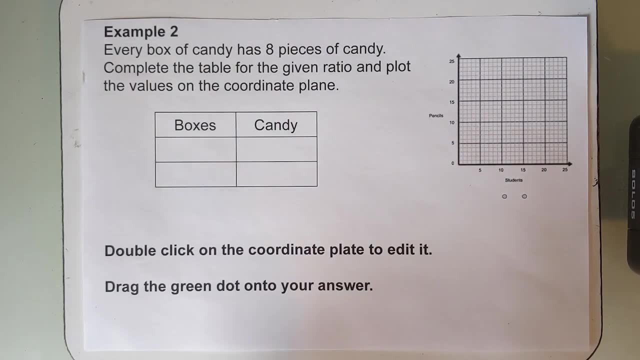 and then we'll go to our coordinate plane in a minute, there right with our ordered pairs. But first we're gonna go ahead and say that for every one box of candy there are eight pieces of candy. So we're just gonna go ahead and fill that out. I'll actually 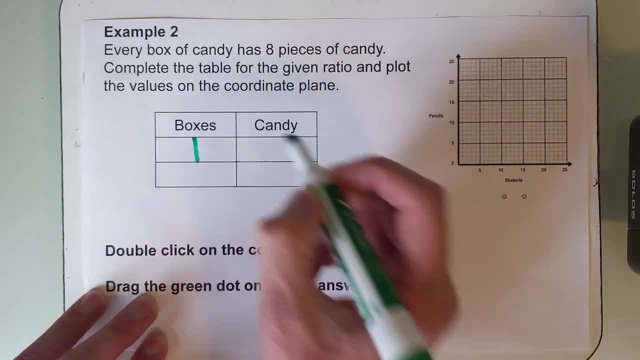 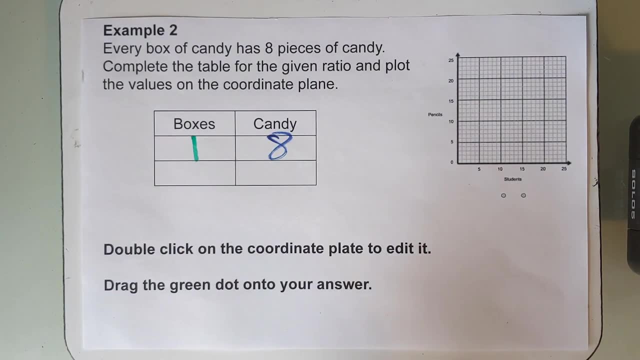 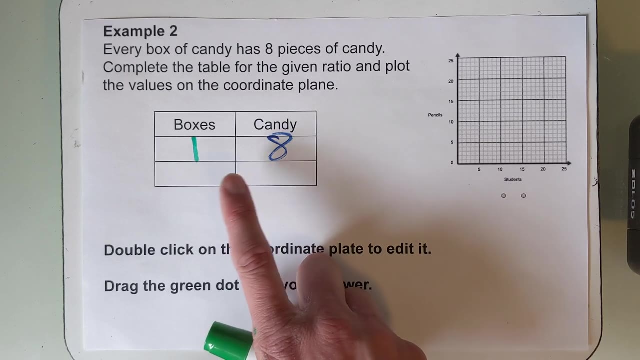 write it down right on here: We have eight pieces of candy, So we have our eight there. Now, thinking again, we're just gonna build on this. We don't have any partial equivalent ratios here. We don't have our candy, We don't have any more in our boxes, So we're just gonna start counting up with. 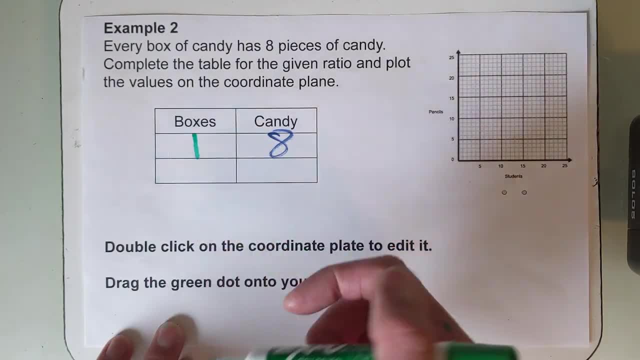 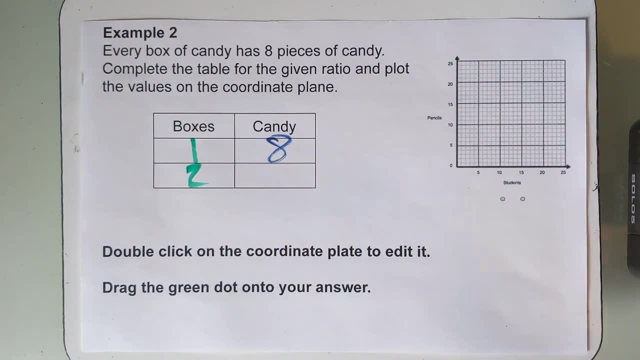 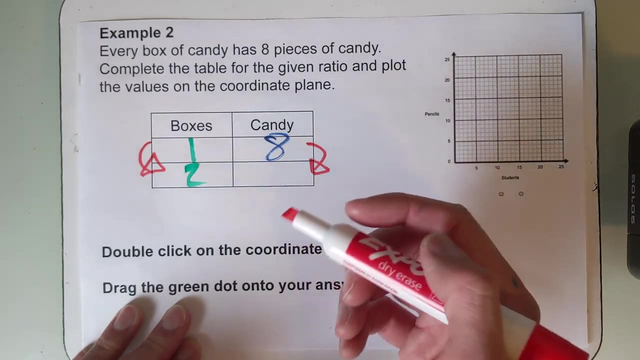 our boxes. So for every one box there's eight pieces of candy. So over here we're gonna go to two boxes and we're gonna go ahead and figure out how much candy would we have there. Now, very similar to our ratio earlier on. our do now our rule is going to think about what our rule is going. 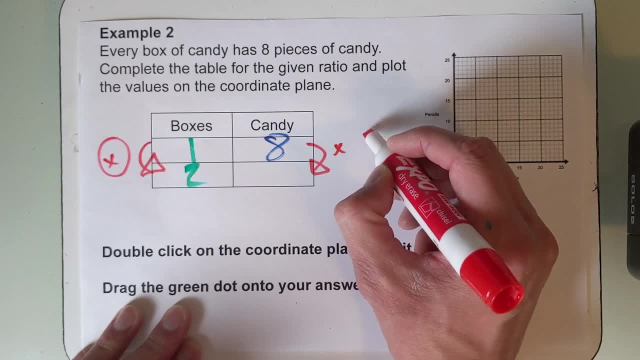 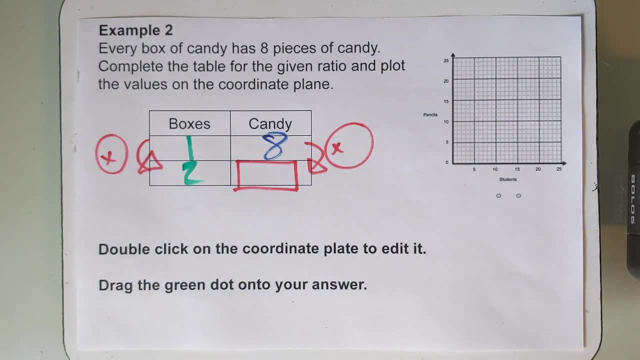 to be. It's gonna be time, something right, And whatever we do to one side, we do to the other. So we're gonna do the same thing there. Go ahead and fill in what you think our answer is gonna be for our candy. Go ahead and do that. I'll give you about 15 seconds. 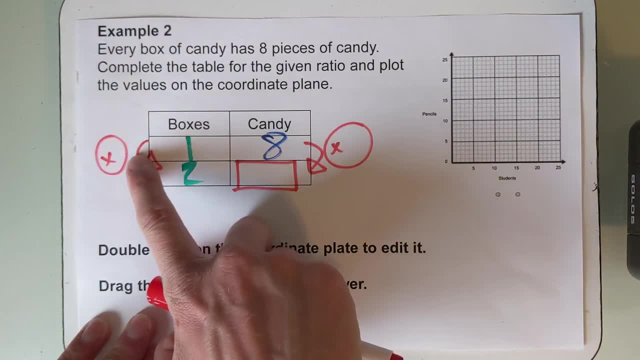 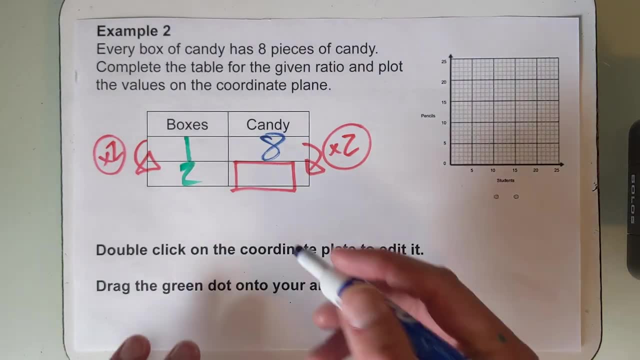 So our rule at this point point is going to be times 2.. So whatever we do to one side, we do to the other. So 8 times 2 is going to give us 16.. So our ratio here is 2 to 16.. Let's go ahead. 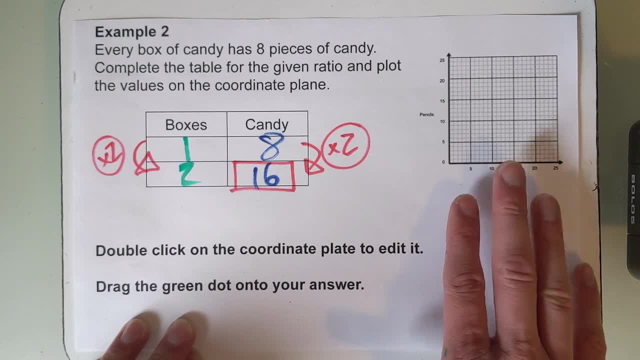 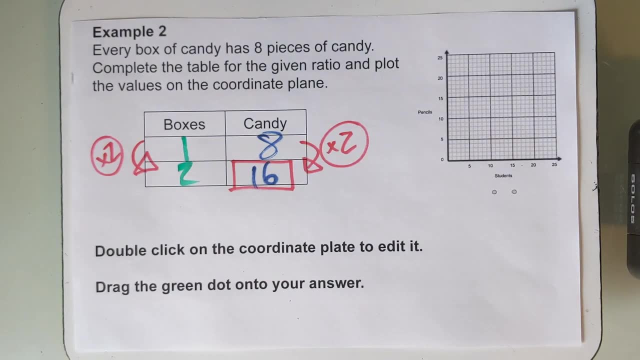 just one more time. We're going to walk through how to actually plot this, and then we will get started on the next question as well. Let's go ahead and take a look at how we would plot this on the computer. So now that we have our table, 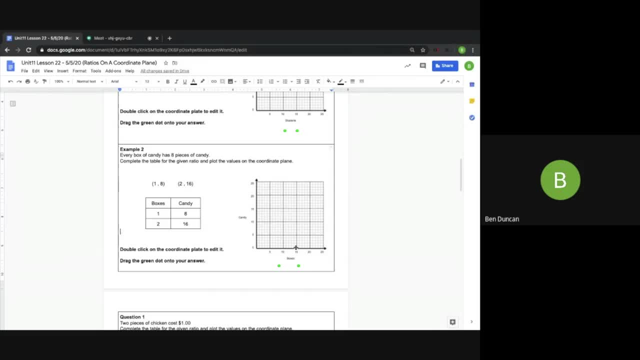 filled out. we're going to go ahead and talk about how to fill in our chart here Just one more time as an example, just like we did for example number one, or I do now. So here again, our ratio is boxes to candy. So our first ratio is: 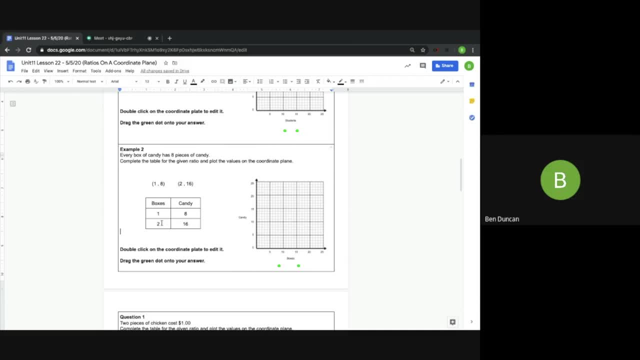 1 to 8. That would be points 1 to 8. And then we have boxes or a ratio 2 to 16. So that would be ordered pair 2 to 16.. So we're going to go ahead and double click on this. 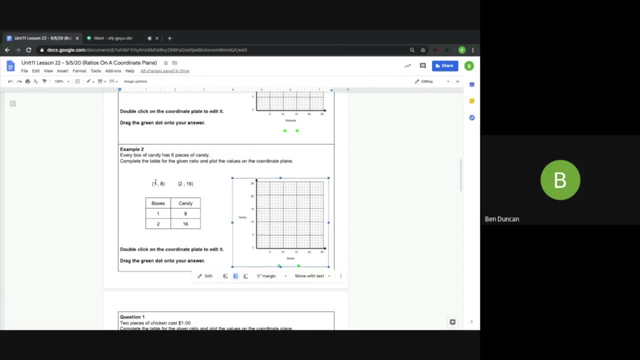 in just a second. And then when we do that, it's going to open it up and we're going to plot our 1 to 8 and then 2 to 16.. So let's just go ahead and double click on it. Remember we go over and 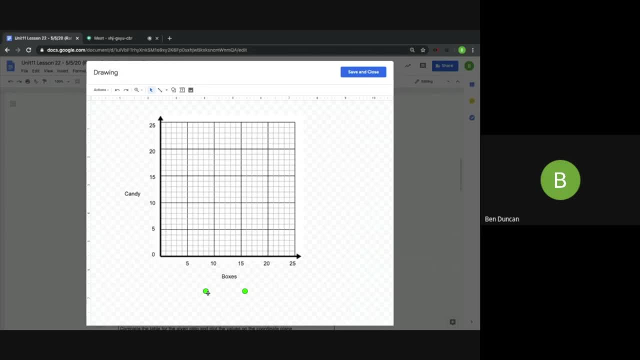 up. You have to walk before you can jump. So we're going to take our first point here. We're just going to grab it and we're going to move it over and from 1 up to 8.. So 1 to 8, right there, First one is there And then we're going to do our. 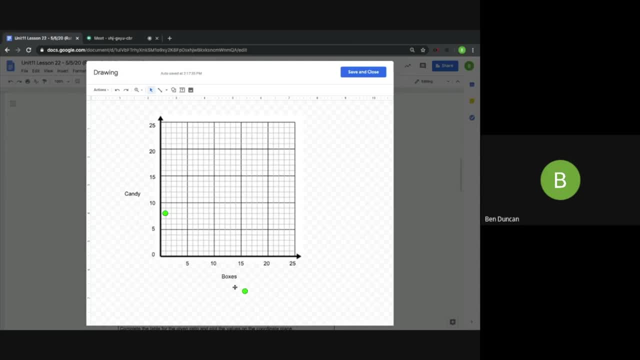 second one, which is 2 to 16.. So remember, over 2 and up 16.. Making sure we're putting it in the right line And we are all set. So we have 1 to 8 and then 2 to 16.. Here we're going to go ahead and press save and close.